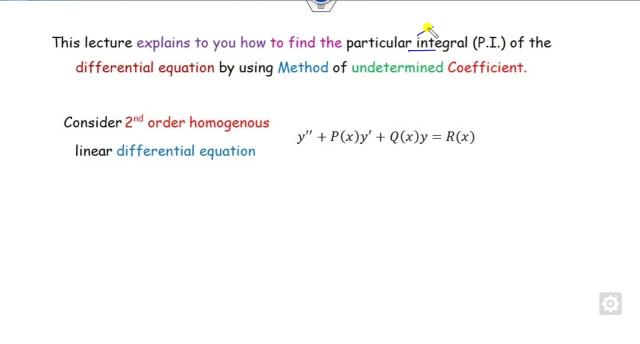 pi by using the method of undetermined. This method is applicable only when this r of x is a non-zero. So whenever there is a r is non-zero, then we can find the solution of this problem- that is, a second order differential equation- by using yc. that is a complementary solution as well as the. 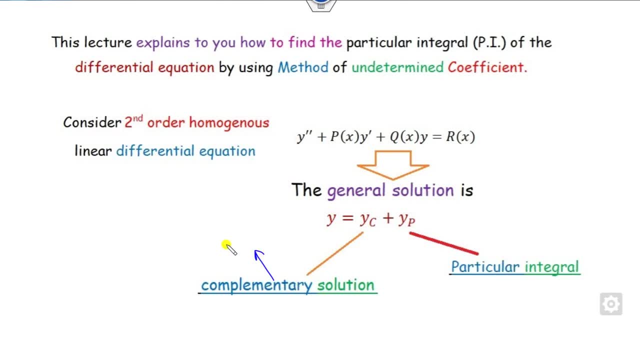 particular integral. We all already knows that how you can find the complementary solution by using the auxiliary equation While this particular integral. you can use this as of the either as operator method, either as a method of the undetermined coefficients, or either you can use as the variation of the parameter. 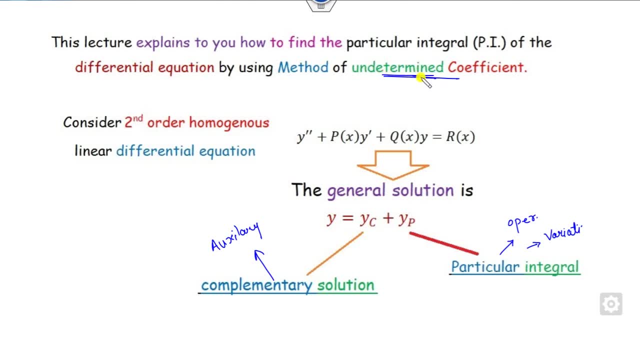 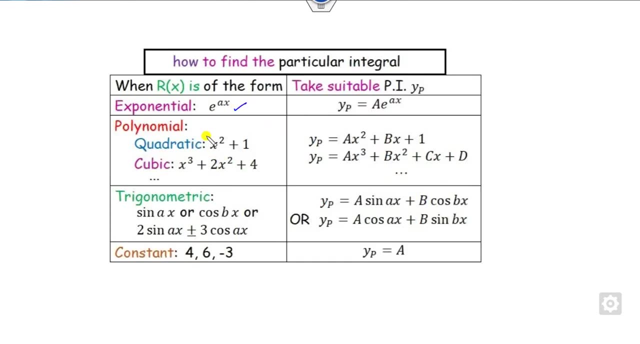 So now in this lecture we will see the method of the undetermined coefficients. So that method is depending upon the nature of this rx, whether this rx is of the exponential form, whether it's a polynomial form, whether it's a trigonometric forms or of the constant forms. are there 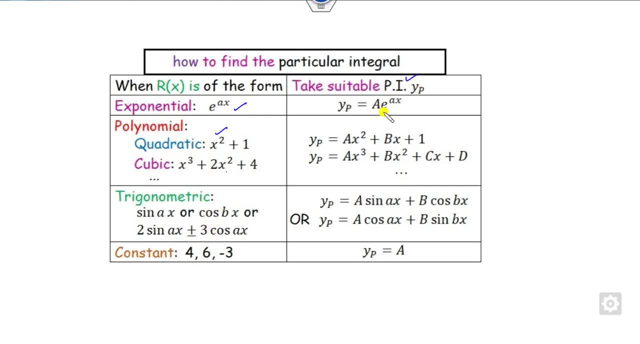 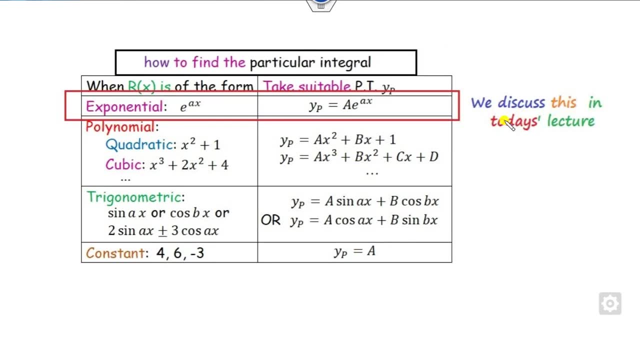 According to their natures. we will take the particular integrals r of here. If it is exponential, we will take as the exponential nature polynomial, then it's a polynomial, and then solve it. So in this here we will discuss only for the first part, while the second third. 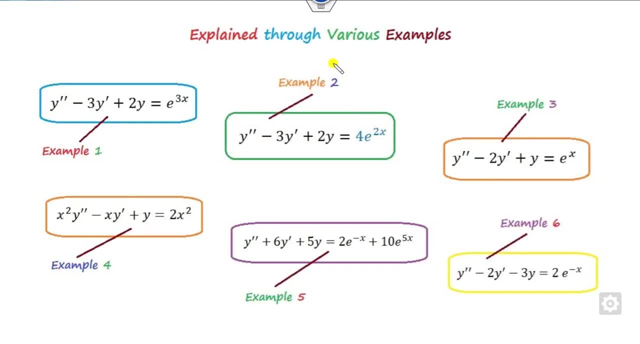 part we will see in the next videos, So we will explain. all these six examples are there. You can see. the right hand side is why this is not the exponential, but we will still solve this one. These all are the exponentials are there and how we can solve this in this video. Myself, Dr Gur. 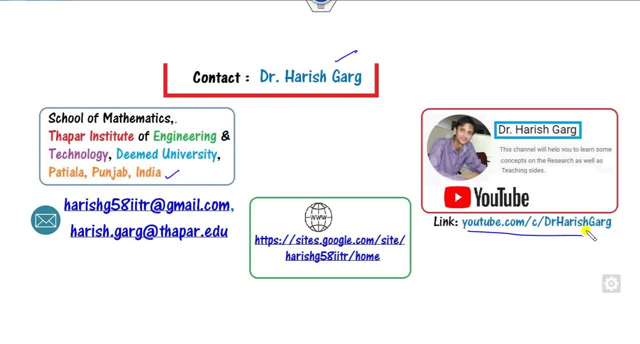 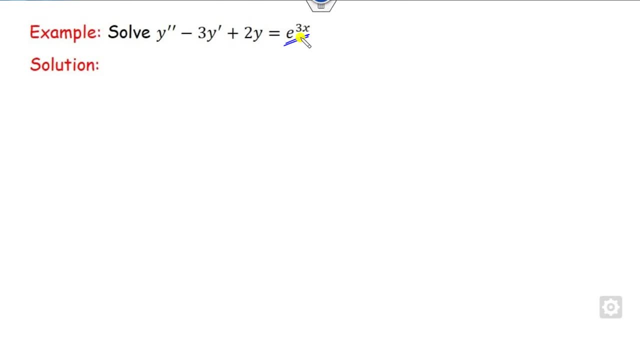 working in the School of Mathematics Thapar Institute. You can simply follow this link for finding the various videos of this differential equations. Now let's see how you can solve this one. So you can see that the right hand side is a non-zero and the coefficients are: 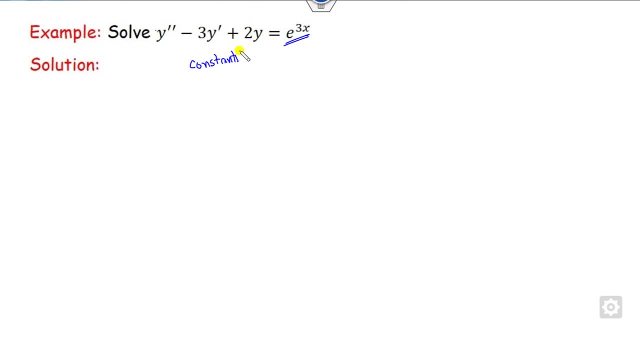 my constants. So you can see the coefficients are my constants. So the general equation of this is written as: y complement y particular. So let's say, firstly find the complement solution. We can write the auxiliary equation as: m square minus 3, m plus 2.. Can you find the roots of this? 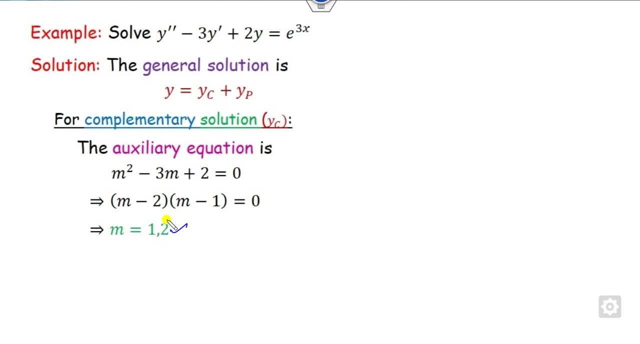 equation. Yes, you can easily find that 1 and 2.. Once you can find the roots, so you can write the complementary solutions as of c1- e raised power 1x, c2- e raised power 2x. or you can say these are: 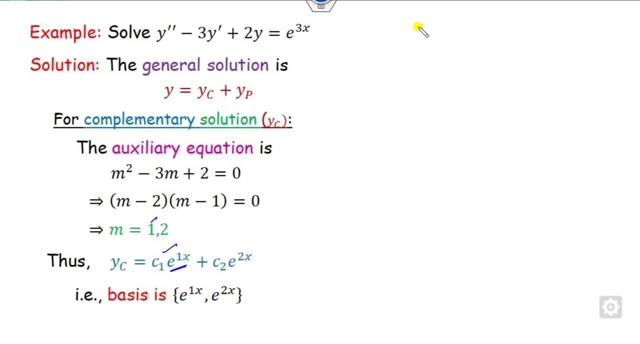 nothing but my bases are there, How you can find the particular integral. Your target is now how I take this one, So forget. firstly, you have to think about that, Since this is my polynomial, this is my exponential are there. so you have to consider the exponential of this nature, whatever it is written, and multiply with 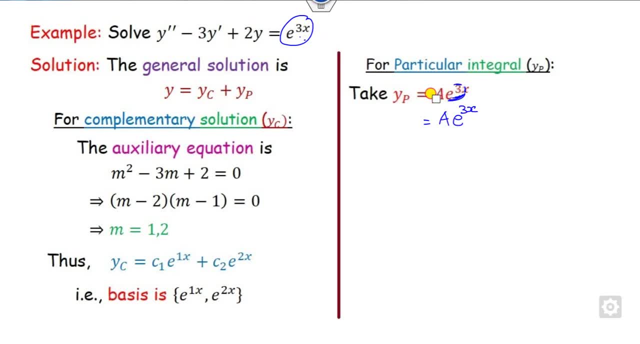 some constant. So that is your target is to find this constant a. are there? Second thing you have to focus on it is that you have to check whether e raised power 3x present in this yc or not. So you have to check whether it is not present. What will happen if it is present we will see in our next. 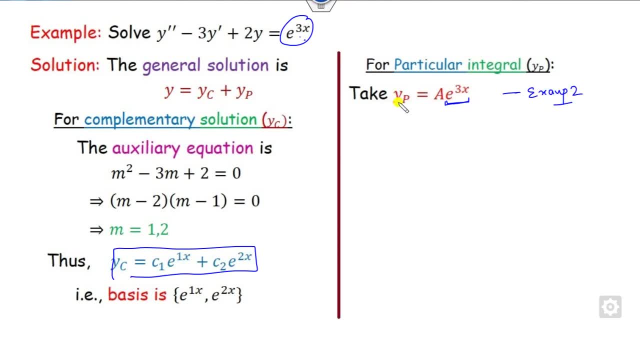 example, that is example number 2.. So now, once it's yp is there, now you have to find the value of the y dash. It is nothing but 3a. e raised power 3x. For that you need the y double dash also You can. 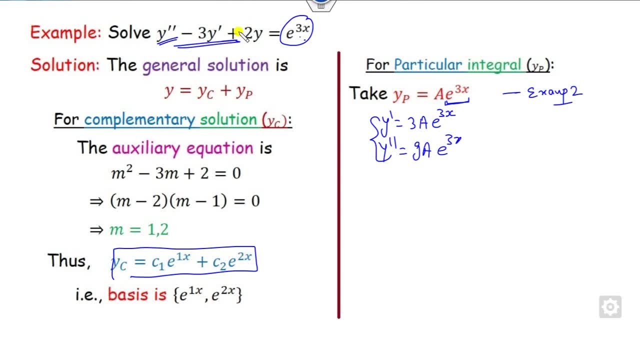 find the value of this. Substitute all these values in here. After solving, you can find the value of a easily. Can you find the value of a easily? Now you can compare them. What will happen? 2 of a is nothing but my. 1. a is my. 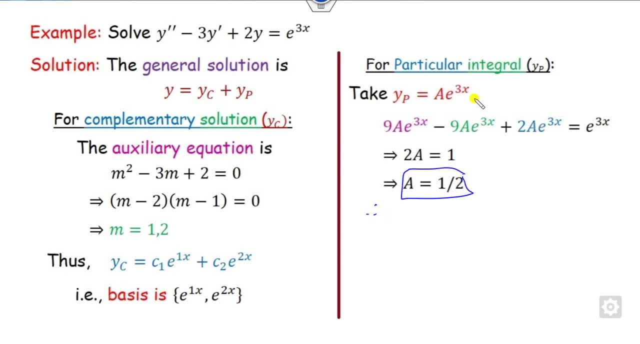 half. So therefore you therefore, once a is half, you can substitute here: yp is nothing but my here. So you can substitute all values of this. yc is my here, yp is this. So the general solution is my here. This is the way you can solve them. Look at the second example where I have you can see that. 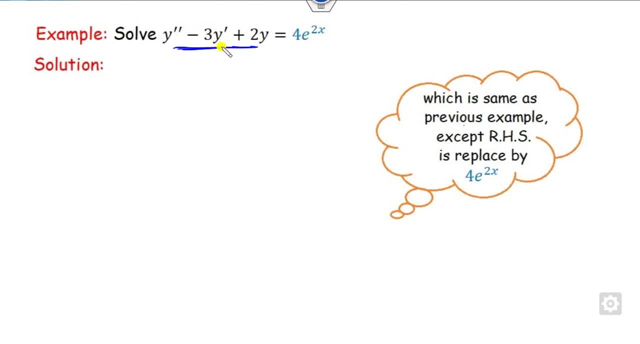 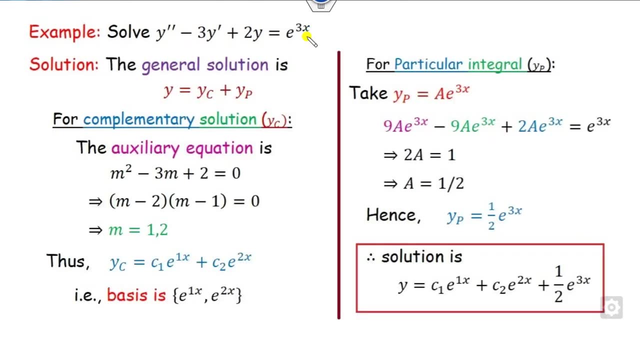 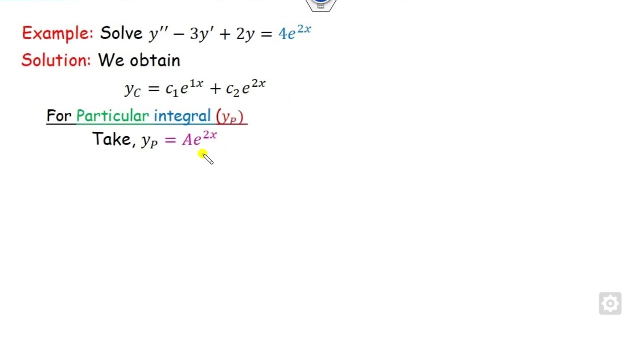 this example is similar as that of the previous one. You can see the right and left hand side is same. I just replace the left. right hand side are there? Again, as we discussed in this same example, you can find the value of the y of c as of this, Now how you can take the y of p. So if I take 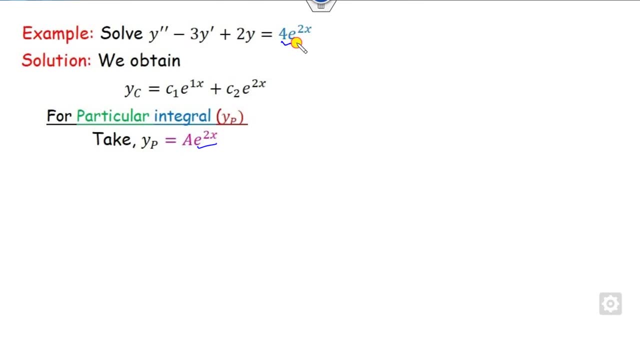 y of p is here, you can see, since this is of here, so I can take as a constant x, e raised power. 2x is also present here. So you can see these two terms are similar because a and c to both are constant. So how you can solve them. So if you try to solve this, you can find the y dash, You can. 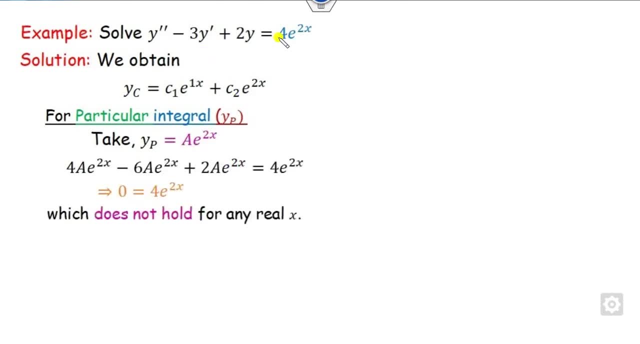 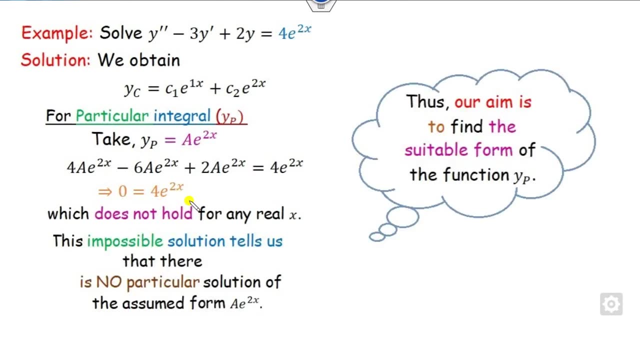 find the y double dash and substitute the value here What you get. You see that 0 is nothing but here. So can you find the value of a from here? It doesn't mean. So what is the meaning of that? This impossible solution tells that there is no particular solution of the form. 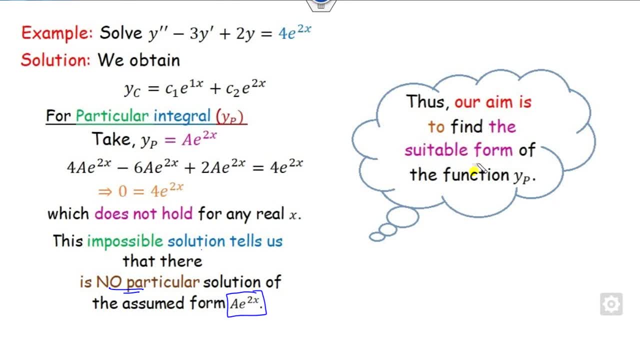 here. So that means our target is to find the suitable form of the function. It means this is not the suitable form. How you can remember that which one is the suitable form? That is depending on this. here You can see that if you take here as a e raised power 2x of this you have 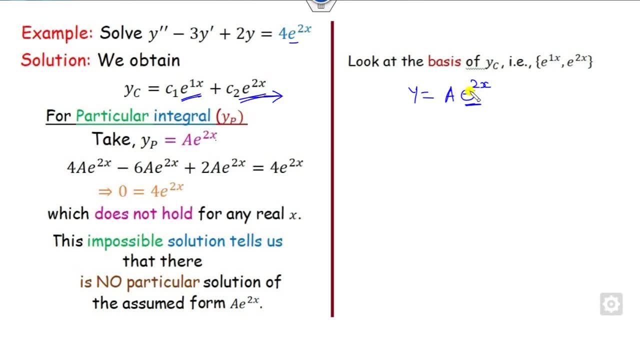 think about this. So you can see that if you take here as a e raised power 2x of this, you have that, whether this is present in the yc or not, If it is present, then how many times it is present? You can see e raised power 2x present one time, So you have to multiply x as a one time, So you 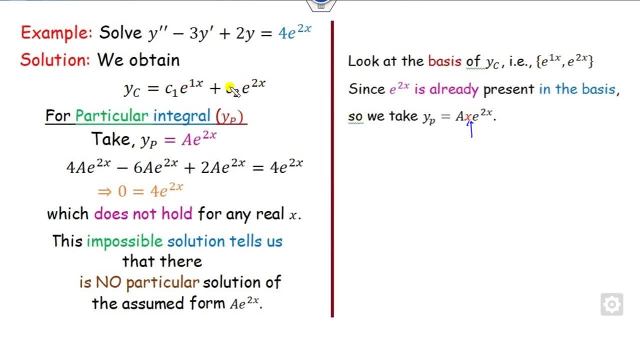 can see that If e raised power 2x present two times, that we will see in our next example. So now you can see this is a e raised power 2x appears one time in the yc So I can multiply this with as a 1x. Now you can find the y dash. You can find the y double dash and substitute. 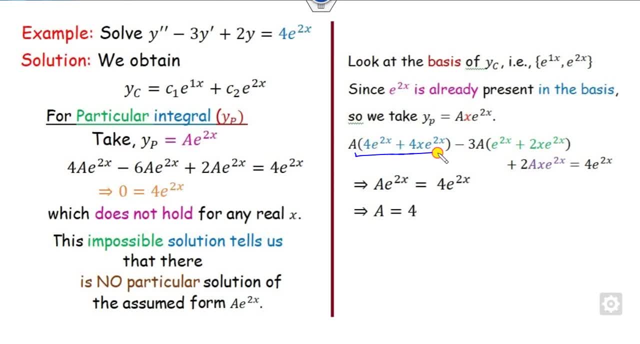 the value again in the given equation. This is the value of the y double dash. This is the value of the y dash and this is the value of y. Now, after the simplify you will get here, Now you can compare the coefficients. A will be my 4.. So what is the value of the? 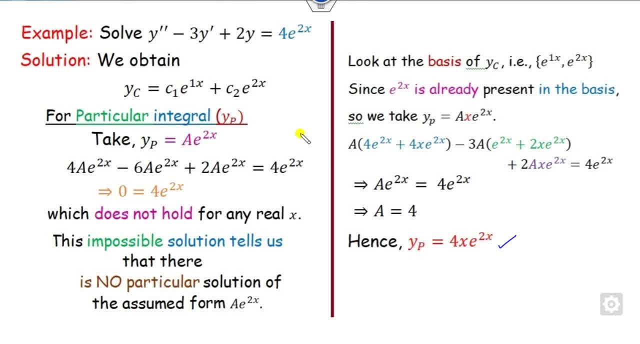 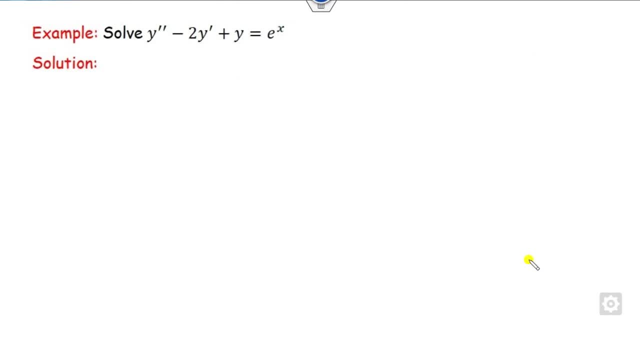 yp Particular integral is nothing but my here, So therefore you can substitute the value in the general solution You will get as the required solution as of here. Look at the another one is there, So you can see again. right hand side is a non-zero, So you can find. 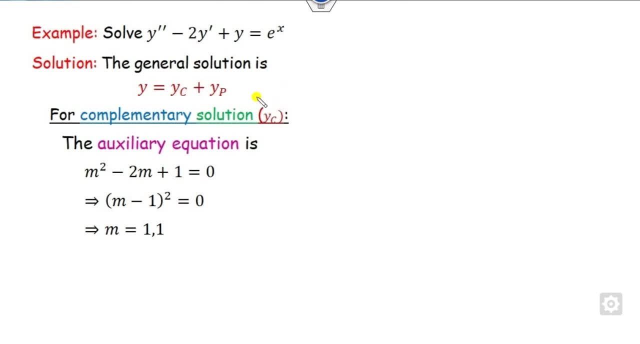 the firstly yc and the yp both. so you can find the auxiliary equation of this like: say m square minus 2m plus 1, you will get here. so what is the value of the yc is now, they are the equal rules. so you can write like of this c1x, c2 and so on, like here, or else you can write: if you write like, 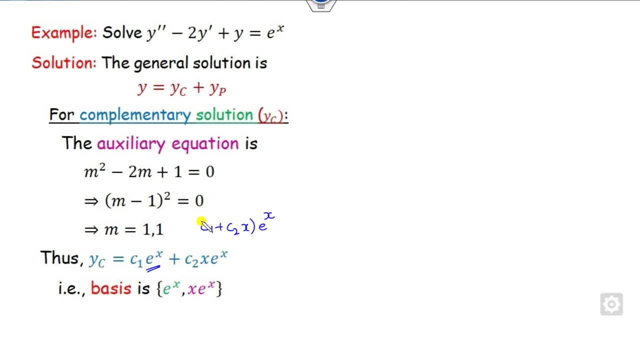 this way you can open the bracket. you can get the same result of here now how you take the, how you take the yp. so since it is of e raised power x, so you have to write e raised power x here. now you can check that e raised power x appears in this or in this how many times. so e raised power x. 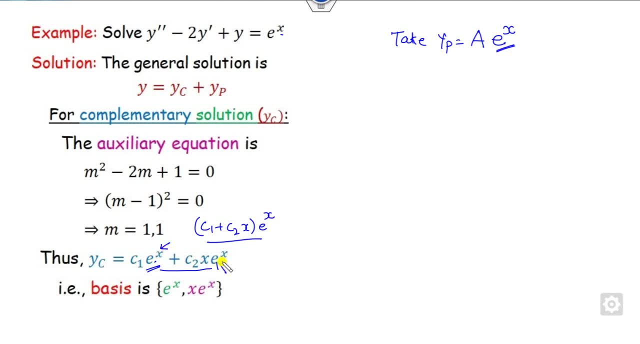 appears two times. e raised power x here. e raised power x also here. so it means you have to multiply this by x square. why? because if if you take this, then it is already present here. if you take only one x, then you can say x into e raised power x is also present here. 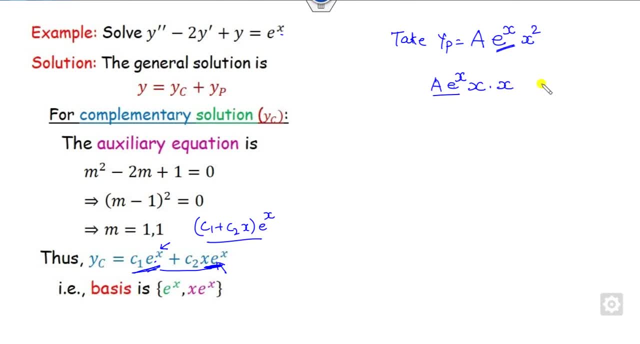 so that means you have to multiply one x more times. so therefore your yp is nothing. but here. now you can take again y dash, y double dash and substitute the value at here you will get: this is y double dash, this is y, and after simplify what will happen, you will get a as of half. so 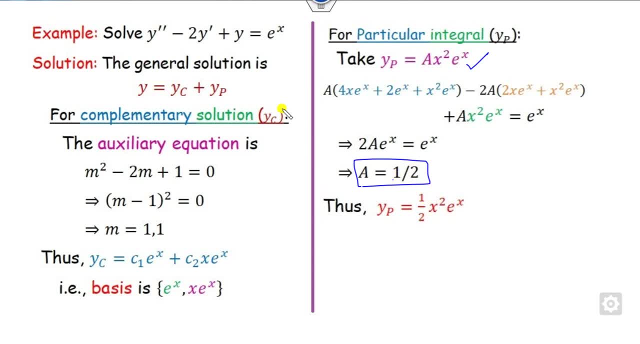 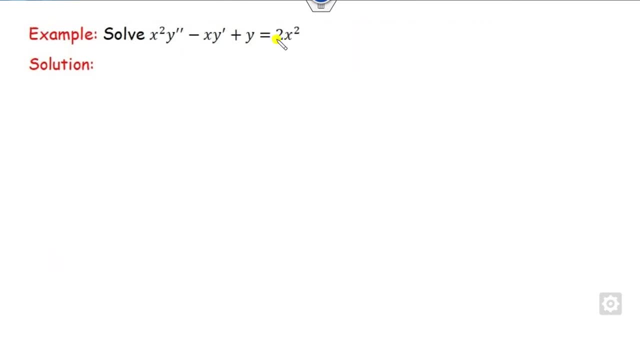 therefore, yp is nothing but my half x square of ex. substitute the value here, you will get the required journals solution. look at this. another example is there. here you can see that the coefficients are not- are not constant. so what is the meaning of that? your first target is to convert this equation. 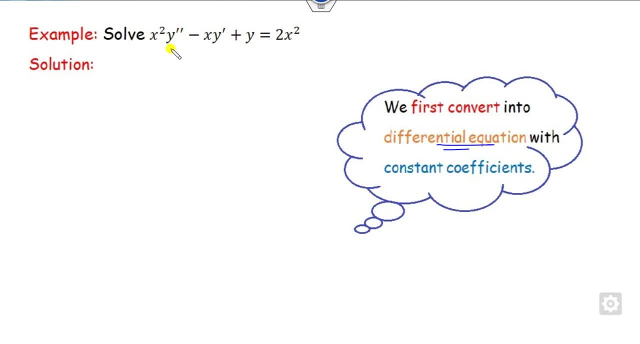 into the constant coefficients. so do you remember that? which one is there? as we discussed in the previous example. what is that? this is nothing but my cauchy eiler equation. why? because x square, then the second derivative one, then first derivative, and so on. so how you can solve. 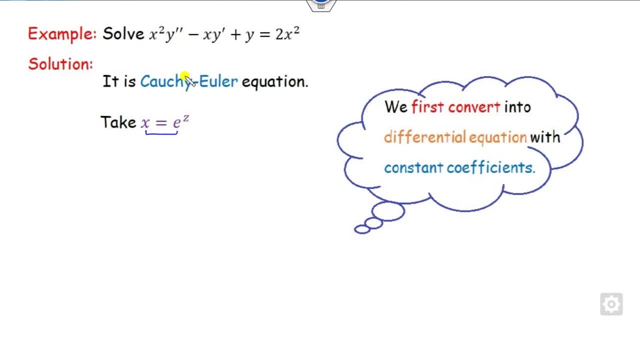 the cauchy eiler equation. you have to take this: x is e raised power z. once it is here, then what is the value of this? this is nothing but the second derivative minus of here. what is the value of the x, y, dash is nothing but. 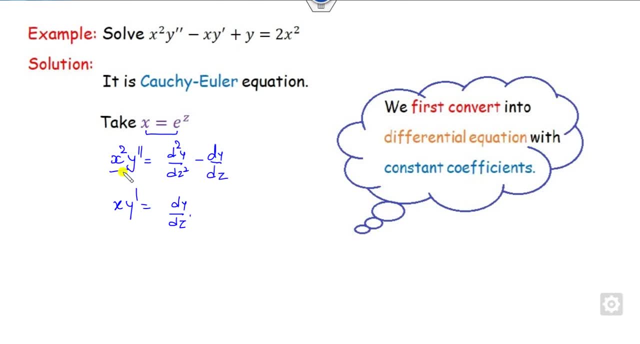 my dy upon dz. now you can substitute these two values into here. what will happen is and x. what is the value of the x? is e raised power, z. now here you can see. this is the constant coefficient. now, right hand side is my exponential parts. are there? now you, we can perform. 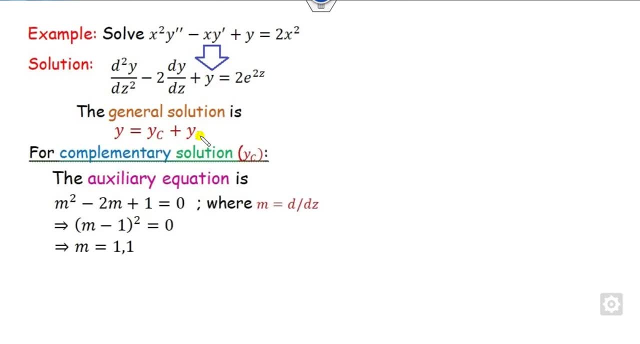 as such. the general solutions are here, where yc's can be written like this way: what is the value of the y? is c1 plus c2. now here m is in terms of the z, so you can write here as of z, e raised to power 2z, so. or you can write like this, this way, here how you can take the value of the y piece, since: 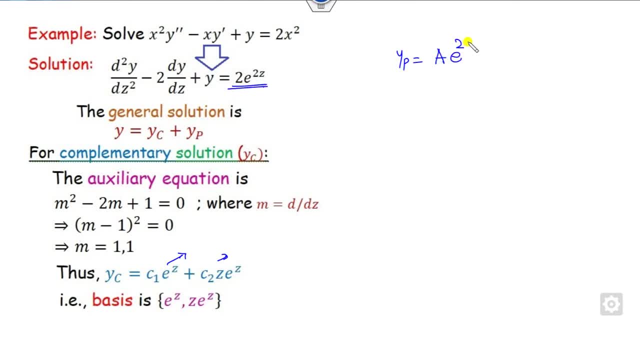 this is my equation. so this is a e raised to power 2z. whether e raised power 2z appears here. no, simply e raised to power 2z appears here. no, simply e raised to power 2z appears here. no, simply e raised power z appears, but e raised power 2z not be appear. so you can take yp as such. so you. 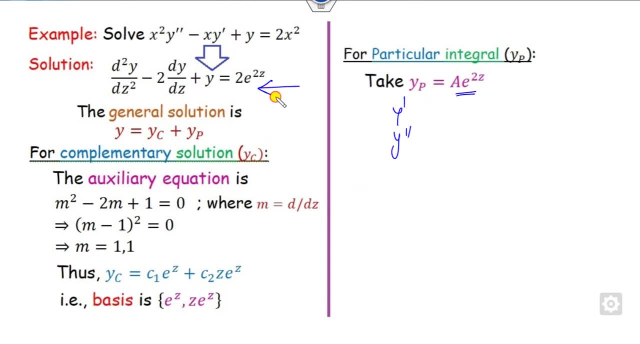 can find the y dash, y double dash. you can substitute this value in here. you will get the expression as of here. a is to yp is nothing but here. so therefore, the general solution of my problem is this one: since z, x, x is my e, raised to power z. so what is the value of the z is? 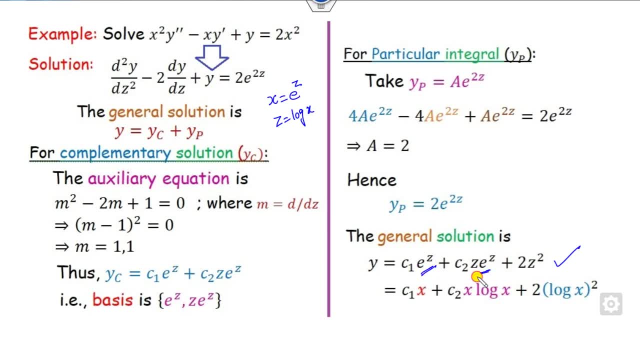 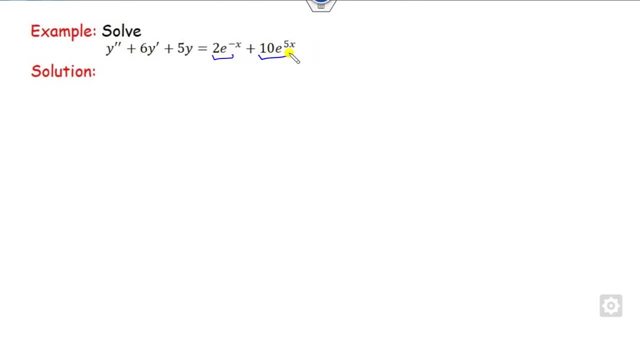 nothing but my log of x. you can substitute the value here you will get the required general solution. look at one more examples. are there? now you can see there are the two exponential terms. are there? so we will firstly find the auxiliary equations m square plus 6, and so on. you can get. 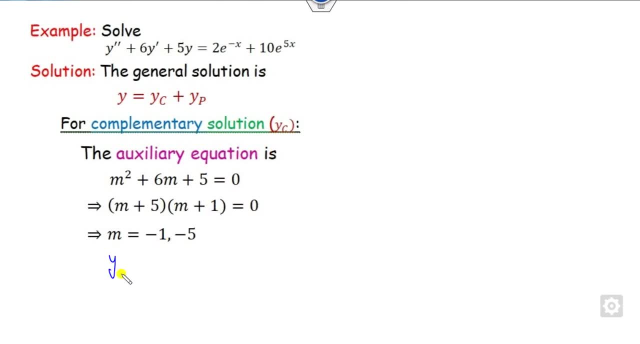 the solutions as of minus 1 minus 5. so what is the yc solutions are there, that is, c1 e raised to power minus 1 x, plus c2 e raised to power minus 5 x. these are here now how you can take the yp is: 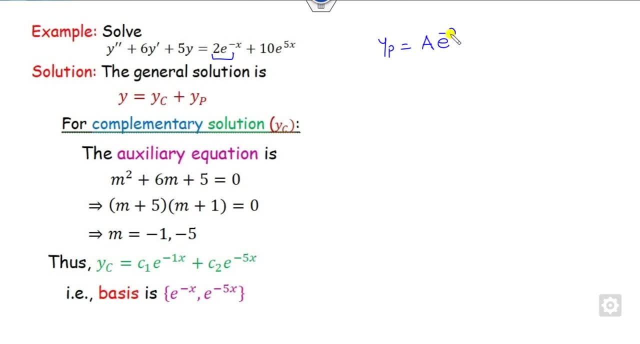 there. so, corresponding to this, it will be my a: e raised to power minus x. corresponding to this, it can be written as e raised to power 5x. so now you can check that whether e raised to power minus x appears here. yes, it appears, so you can. how many times appears. 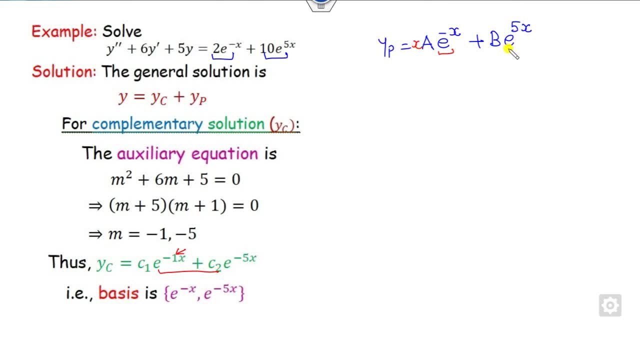 only one time. so you have to multiply this by x, whether e raised to power 5x appears here. no, e raised to power minus 5x appear, but plus is not be there. so there is no need to multiply x. so what is the yp? is my x a x, e raised to power minus x, and so on. rest part is similar. 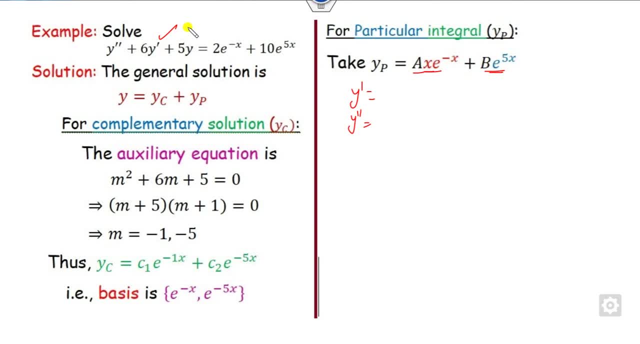 so you can compute the y double dash, y dash. substitute the value here you will get after. simplify you here. now you can equate the coefficient of e raised to power minus x. you can equate the coefficient of e raised to power 5x, and now you can equate them here. definitely, this will be. 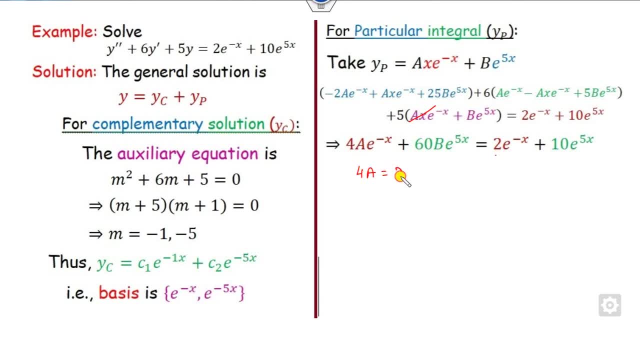 cancelled out if you open them. so what is the value of this? so what is that? 4 of a is nothing but 2. 16 of 60 of b is nothing but my 10. so you can easily find the value of a and b here, so once. 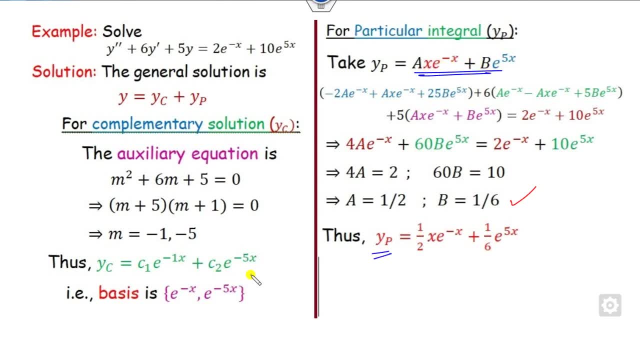 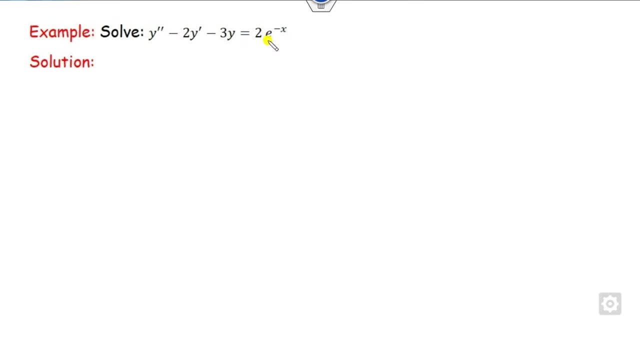 b are here. you can substitute this. yp is here, yc is my here. so the general solution is my here. look at the last example. so here again, the right hand side is my exponential part. you can find the auxiliary equation here. so can you find the roots of this? you can easily find.